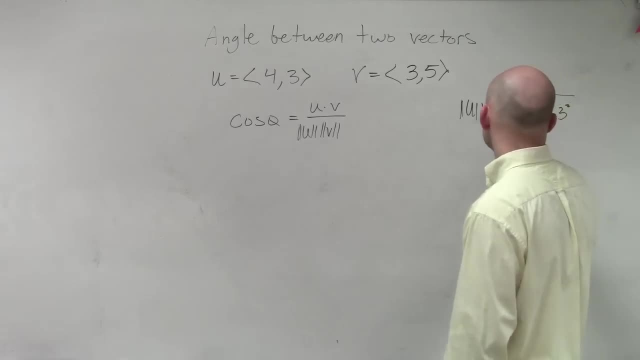 Yes, Okay, So we go. 16 plus 9 is going to be 25.. So that equals 5, right? Then let's do the magnitude of v. Magnitude of v is going to be the square root of 3 squared. 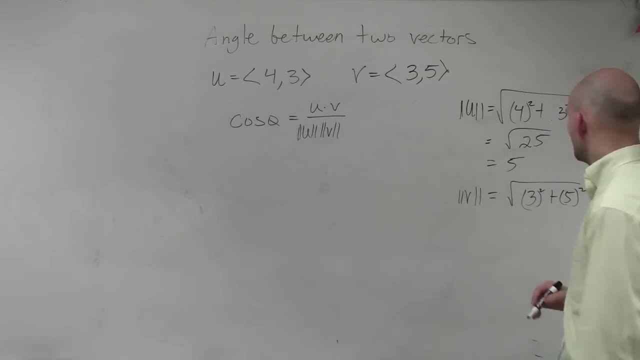 Plus 5 squared, So we'll have 9 plus 25 is going to be the square root of 34, right, Okay, Then let's do the dot product of u times v. Dot product of u times v is going to be 4 times 3 plus 3 times 5, which equals 12 plus 15,. 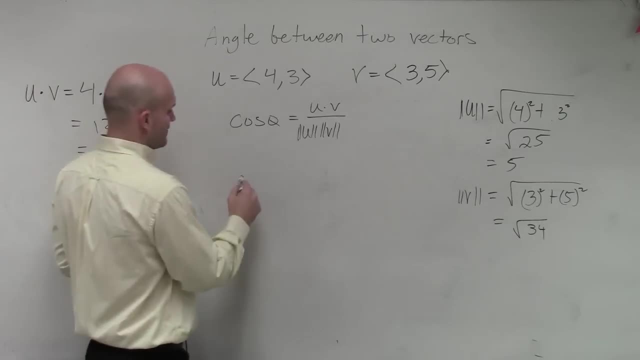 which equals 27.. So therefore I have: cosine of theta equals 27 divided by 5 times the square root of 34.. Now we look at this and we say: can we simplify anything you know to make this a little bit easier? 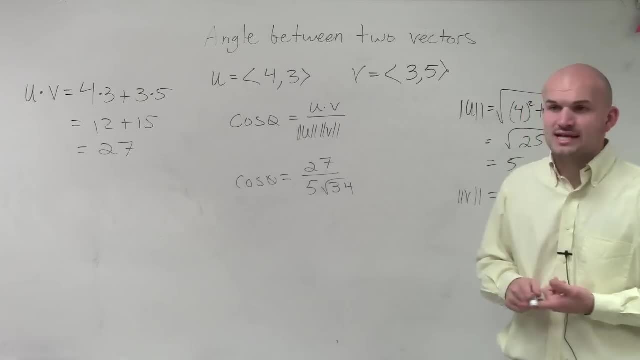 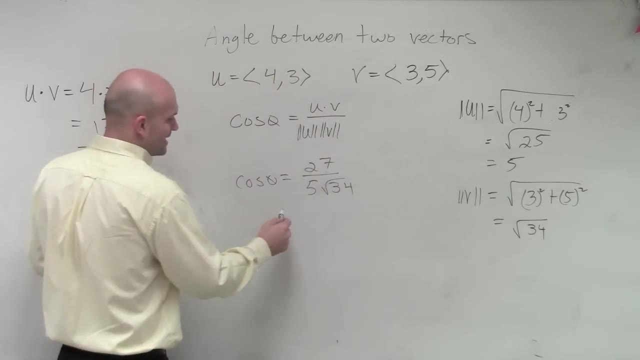 Can we simplify the square root of 34?? Can we reduce anything between 25, 27 over 5?? No, really nothing. So to find theta, I can say: theta is going to equal The cosine inverse of 27 over 5 times the square root of 34.. 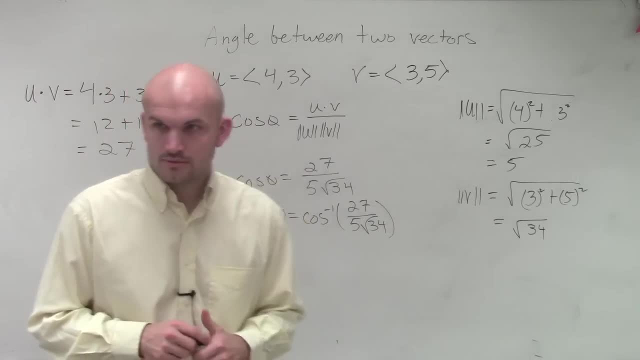 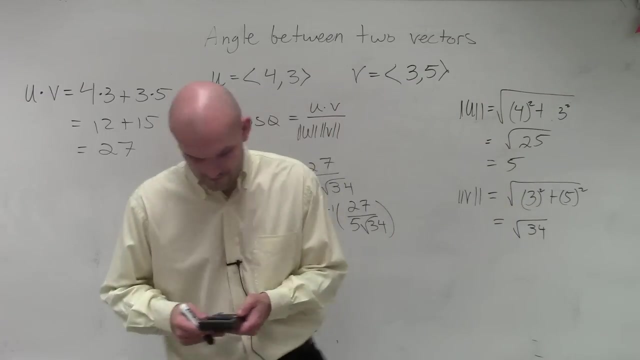 So now I need to figure out what that value is, So I'll use my handy calculator, donated by a student who had to go to the restroom. 22.2? Okay, So much for that video. now, Okay, Inverse cosine. 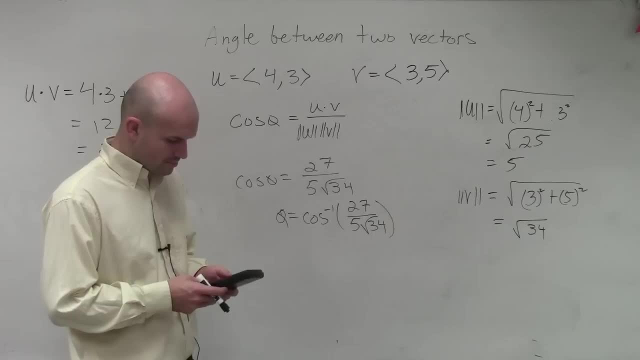 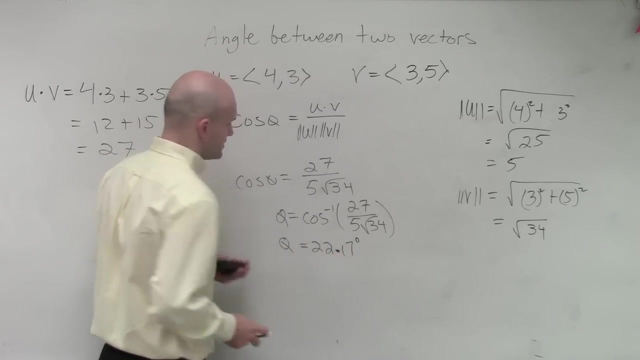 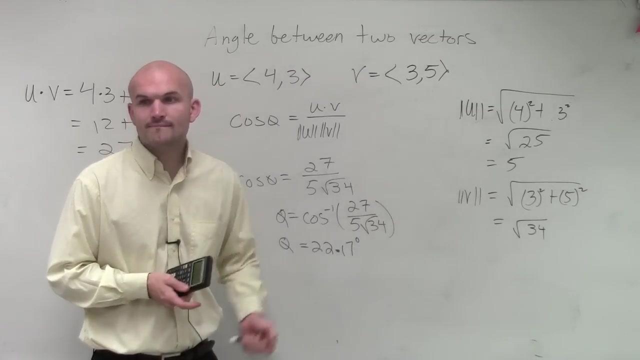